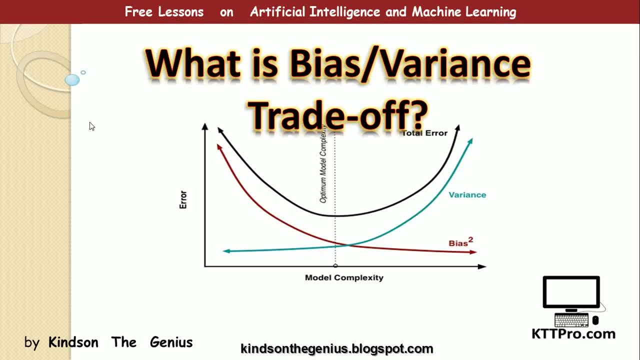 Hello, I am Kainz on the Genius and today we are going to be talking about bias variance trade-off in machine learning. Bias variance trade-off is a very important topic in machine learning and that is what we are going to discuss today. I just want: 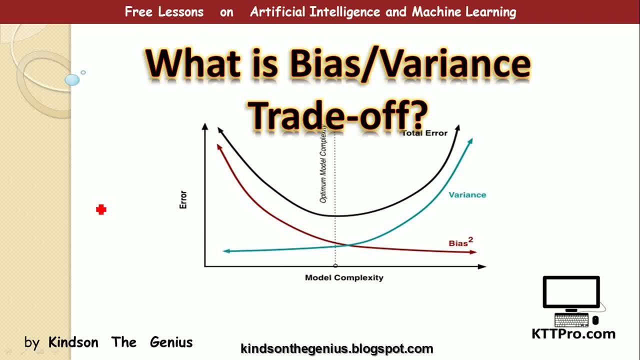 to remind you to please subscribe to my channel. Just click on the subscribe button there, and that will enable me to make better videos next time. So please subscribe now. click on the subscribe button so that I make better videos for you. Alright, so presentation for this. you can print it out from this place. kainz on the. 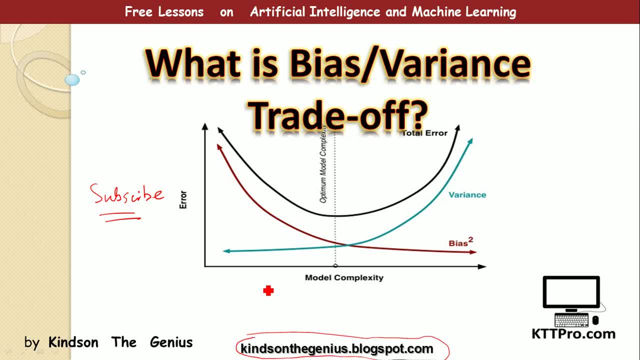 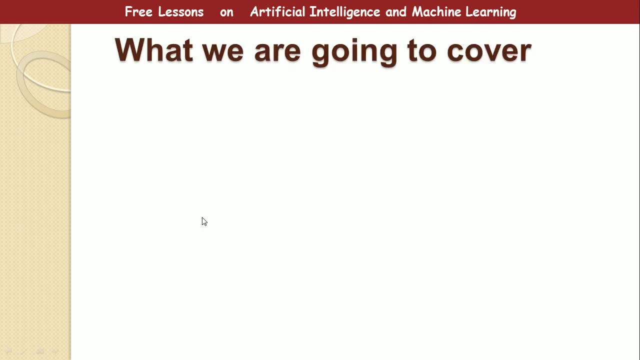 geniusblogspotcom or hu For this particular presentation. the link is in the description box, so you can just click to download the presentation and then you can read. you can print. Alright, so let's get started. What are we going to cover today? We are going to look. 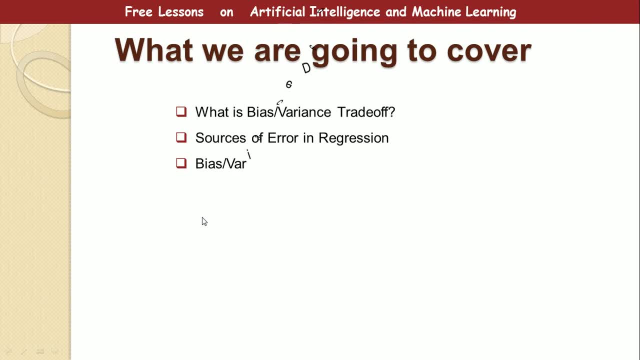 at what is bias variance trade-off. We are going to look at sources of error in regression: bias variance, decomposition of squared error, trade-off, minimizing the error, the relationship to under-fitting and over-fitting. We are going to illustrate it or demonstrate it: The bias variance trade-off graph: we 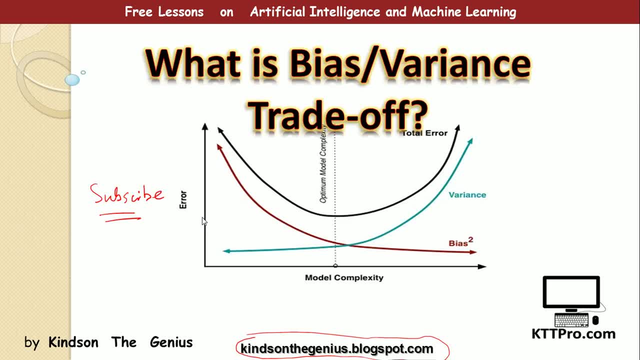 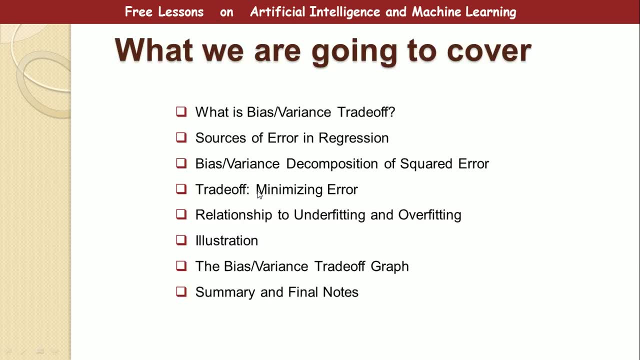 explain it. That is the same graph you saw in the initial part. This graph- this is the bias variance trade-off graph- Very important. We are going to explain it along the line And then we summarize and discuss a few final notes. 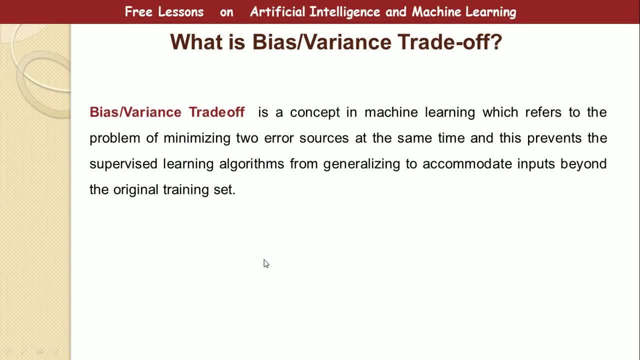 So what is bias variance trade-off? Bias variance trade-off is a concept in machine learning which refers to the problem of minimizing two error sources at the same time, and this prevents the superlative from being eliminated if the error doesn't remain at the same time. 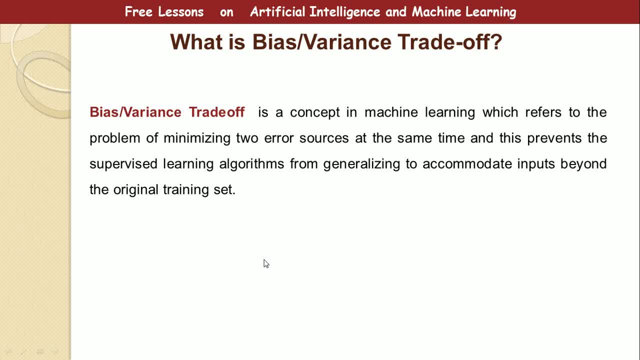 prevents the supervised learning algorithm from generalizing to accommodate inputs beyond the original dataset. All right, let's break this down. For the initial part, take note that we need to minimize two errors at the same time. These two errors are the bias error and the variance error, so we want to minimize it. 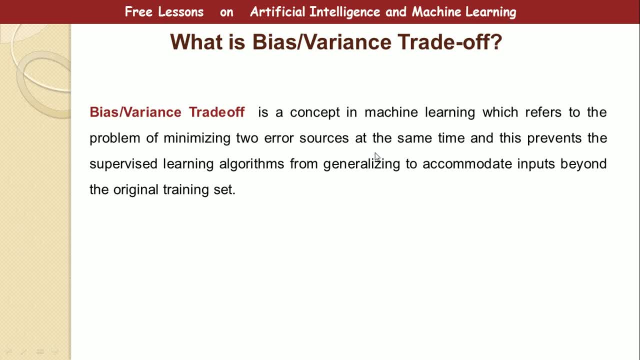 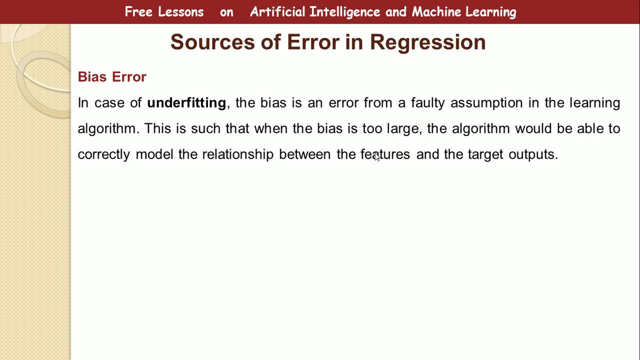 at the same time, but we prevent going too far so that it will affect the algorithm. So the two error sources are the bias error and the variance error. We are going to minimize these two errors at the same time. So what is bias error? 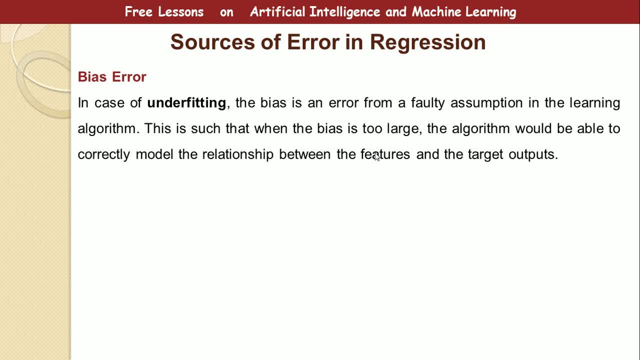 Now, bias is an error from a faulty assumption in learning algorithm. okay, This is such that when the bias is too large, the algorithm would fail. Okay, The algorithm will be able to model the relationship between the features and the target variable. Actually, there is an error there. 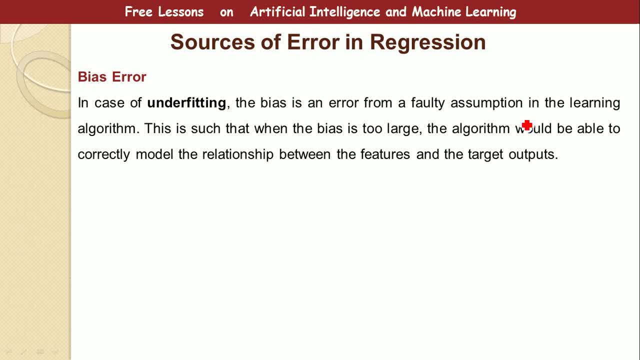 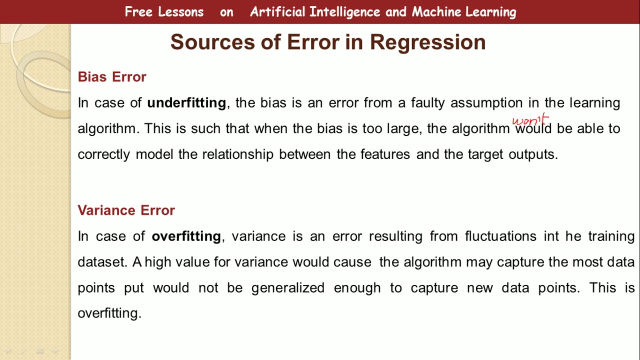 When the bias is too large, the algorithm won't be able to correctly model relationship between the features. So that is, when bias is too large, all right. So when variance error results from fluctuation in the training dataset, okay, a high variance. 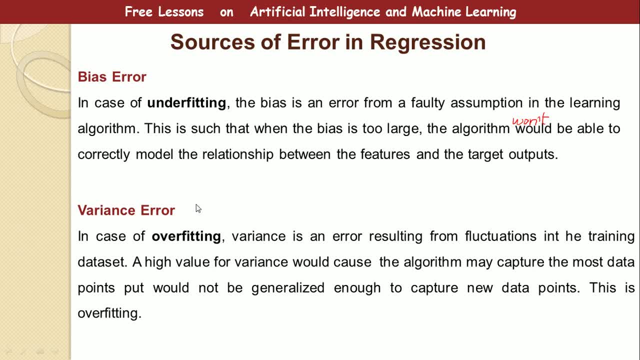 value will cause the algorithm to capture most data points, but to not be generalized and not to capture new dataset. Let's just illustrate this. I'd like to. I'd like to make some drawings on the screen. So let's take, for instance, we have something like this: 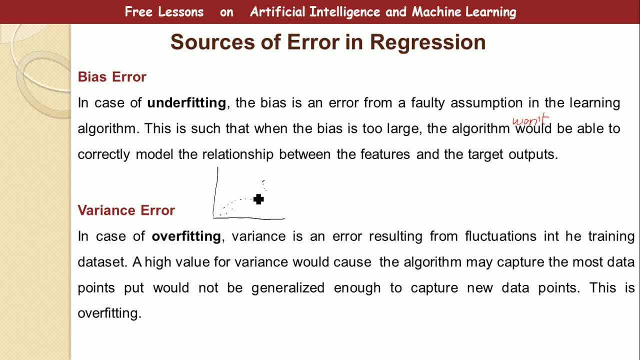 You have data points in this way? Okay, so now, if the bias is too large, then the algorithm won't be able to model the relationship. maybe we can now have something like this. So in this way, you see, the data points are not actually captured. 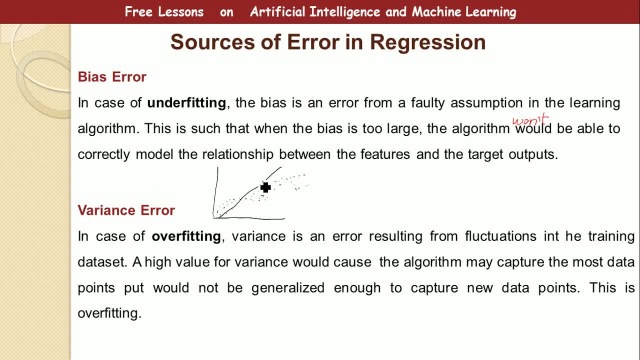 So this is called underfitting, where the bias is too large. In this case, the algorithm does not capture or does not model the relationship in the correct way. On the other hand, Variance error is when the variance is too high. okay. 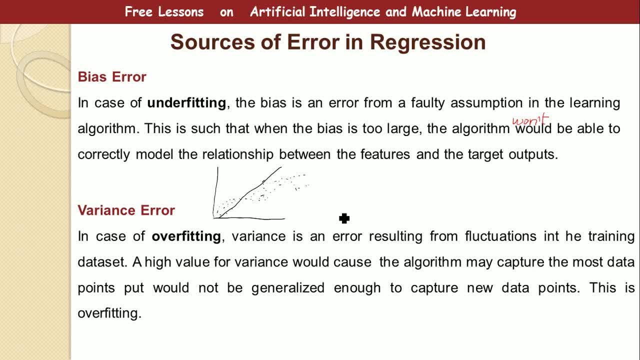 In this case the algorithm will capture most of the data points, but will not be able to model or capture new data sites. Let's illustrate in case of a high variance error. So in this case the algorithm might be something like this: Capture all the data points. 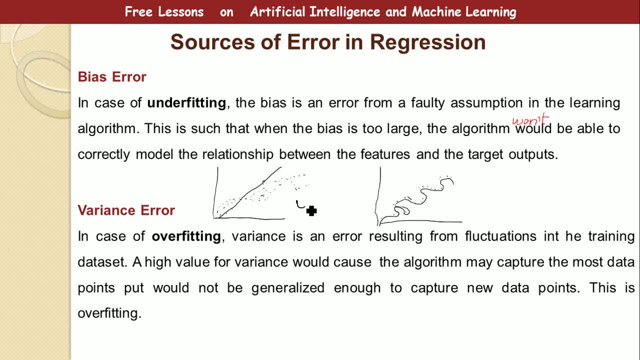 So in this case, in the case of the bias being too large, we have underfitting, and in case of variance being too high, we have overfitting. So how do we adjust these two errors such that we don't get into overfitting or underfitting? 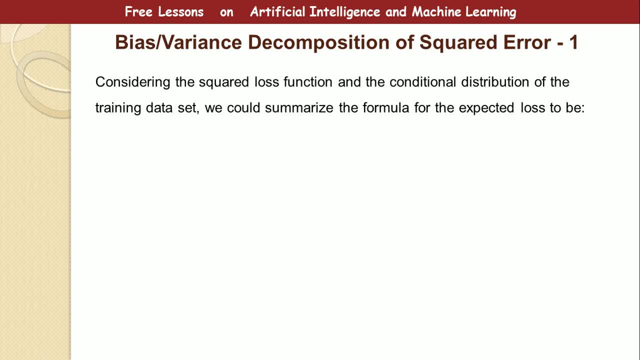 In this case, we now have to talk about the decomposition of the structure. Okay, So we need to know that the expected loss in the model is given by bias squared plus variance plus noise. So, assuming that y output is equal to function of x, representing the relationship between: 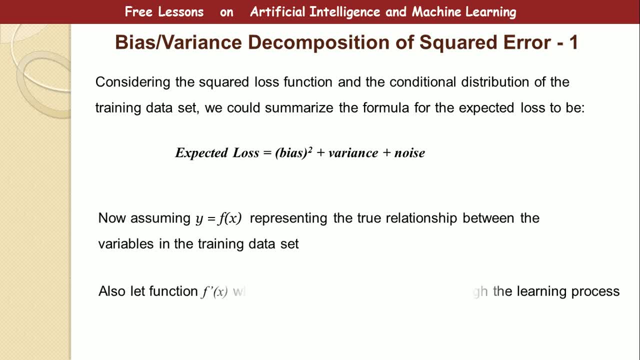 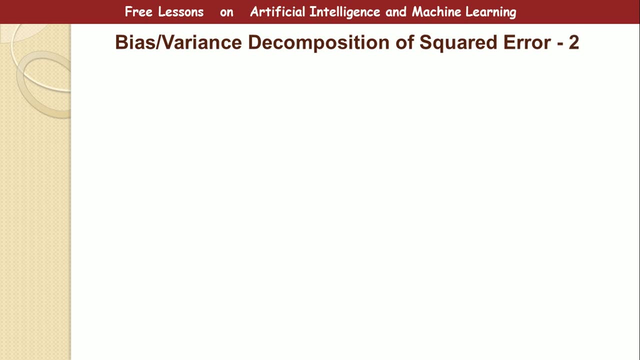 the two: the input variable and the training data site. then f prime of x is an approximation, which is actually the input variable. Okay, So f prime of x is the output from the algorithm. f of x is the actual output, f prime is the. 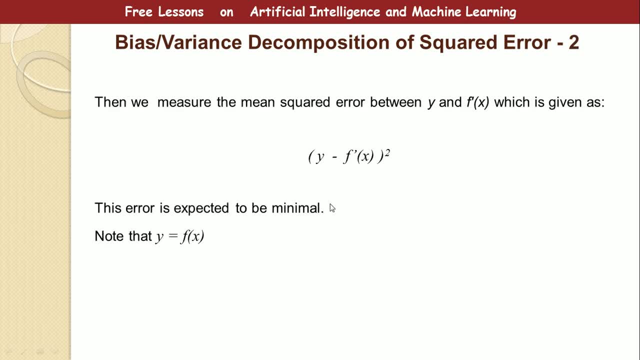 output from the algorithm. So now we measure the squared error as y minus f prime of x. So you see that f prime of x is the measured value and the actual is y. So this is actual. This is the measured or the output from the algorithm. 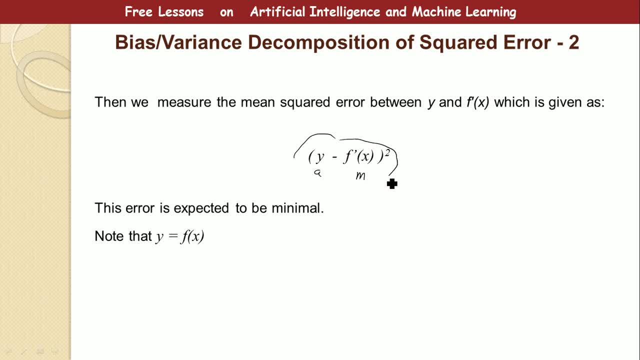 So we want to keep this error minimal. we want to keep this error to be minimal. So we know that y is also equal to f of x. Let's now decompose this error into bias, variance, noise and other things. So we have y minus f of x squared. the squared error is equal to bias. 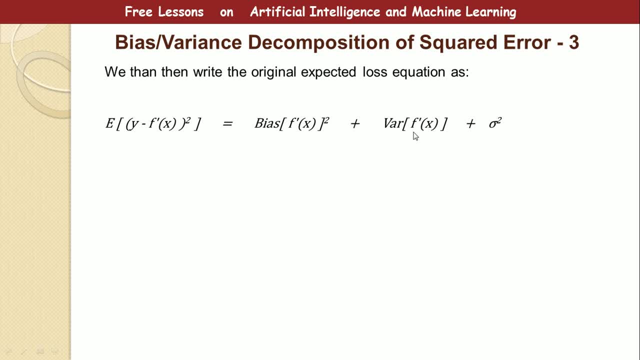 So we have bias squared, variance squared. sorry, variance plus the noise. This value represents the noise. where we have that bias is equal to the output from the algorithm minus the actual value. Variance is given by the formula for variance: this squared minus this, all squared, and then 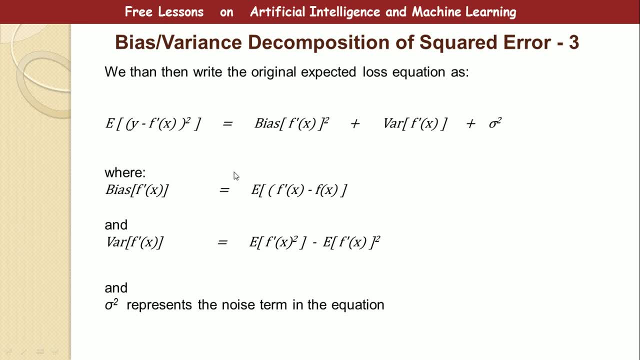 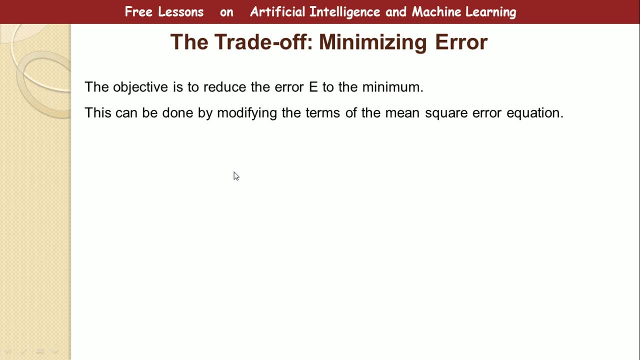 this represents the noise term in the equation. So now, what does the trade-off has to do? The objective is to reduce this squared error to the minimum. To be able to reduce it, we are going to modify the terms of that equation, which means that 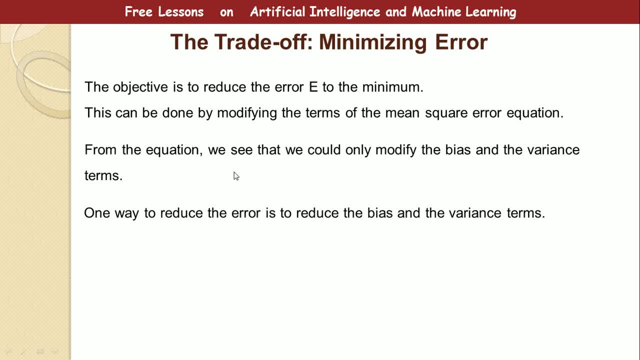 we are going to either reduce the bias, reduce the variance or reduce the noise, because these are the three terms in the equation. But we can only reduce either the bias or the variance. We cannot reduce the noise Now. we cannot reduce the bias and the variance simultaneously. 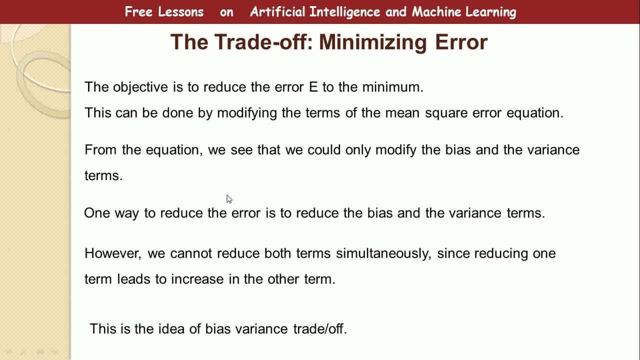 So the key word to take note of here is: you can't reduce the both of them. you can't reduce the both of them simultaneously, Because if you are reducing the bias, the variance is increasing. If you are increasing the variance, the bias is reducing. 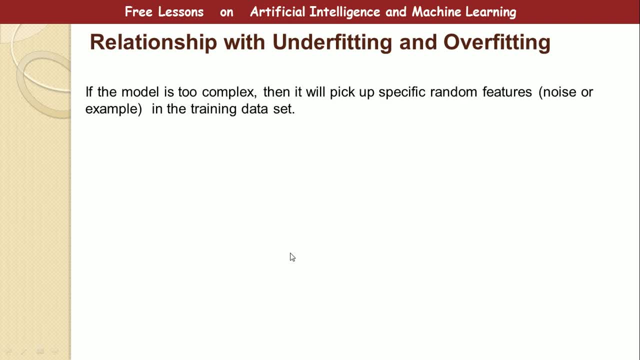 All right. so let's now see the relationship between bias-variance, trade-off and overfitting or underfitting. I have mentioned before that if you are increasing the bias, it will lead to underfitting. On the other hand, if you are increasing the variance, it will lead to overfitting. 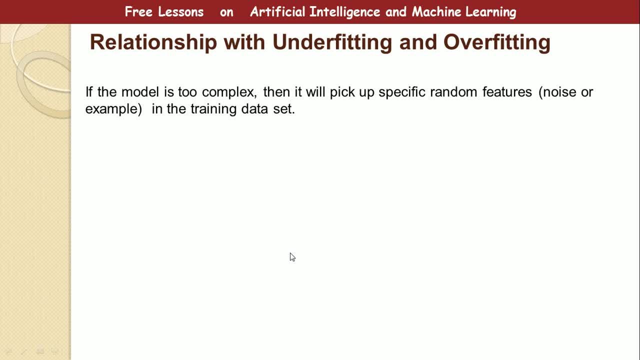 Meanwhile, if you are increasing the bias, the variance for sure you will be reducing. If you are also increasing the variance, the variance will be decreasing. So this is what we are going to do. So these are kind of intricate, completely intertwined relationship between these two. 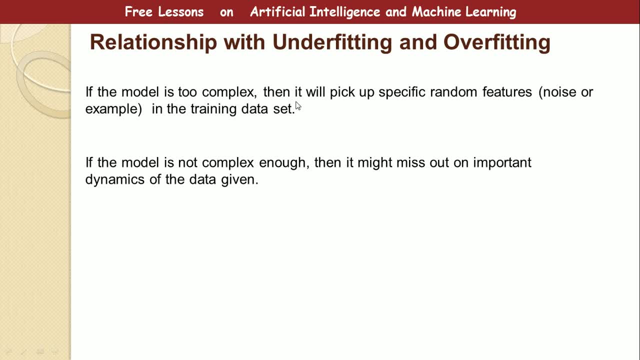 concepts. If the model is too complex, meaning that there is too much variance, then it will pick up specific random features or noise from the example in the training data set. So when we illustrate it, we see that when the variance is too high, when the variance 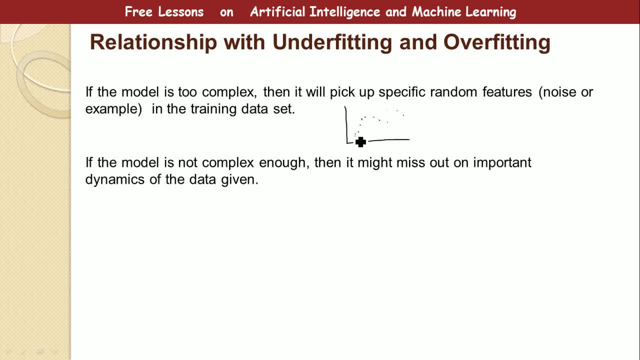 is too high, it's going to pick up the overfitting. All right. So if the model is too complex, everything is going to pick up everything, including even the noise in the data. Now, if the model is not complex enough, that is, there is no enough variance, it will miss. 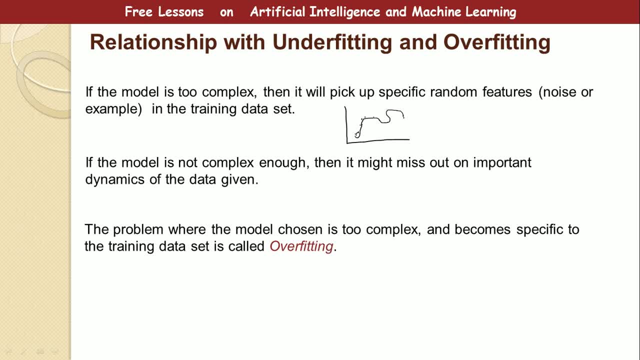 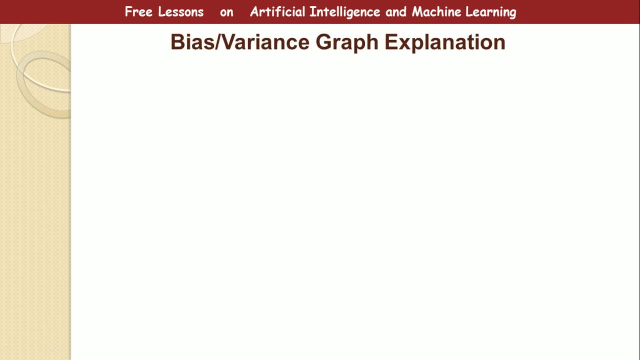 out on important dynamics of the data set. When the variance is too complex, it's called overfitting, But when the model is not complex enough, it will miss out on the important dynamics of the data set. When the model is not complex enough, it results to underfitting. 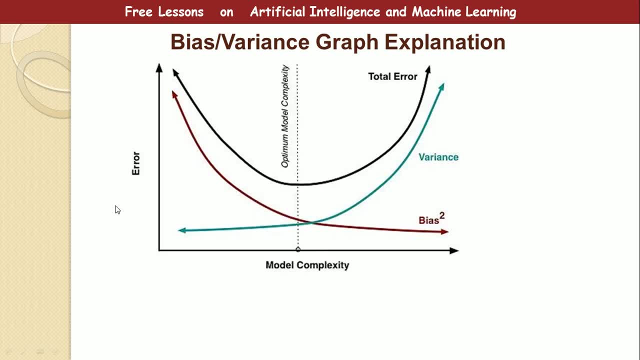 Let's look at the graph now. Now pay attention to this graph, because it's very, very important. This is actually the graph, the main graph, that highlights the bias-variance trade-off concept. Now, the red line is for the bias, The blue is for the variance. 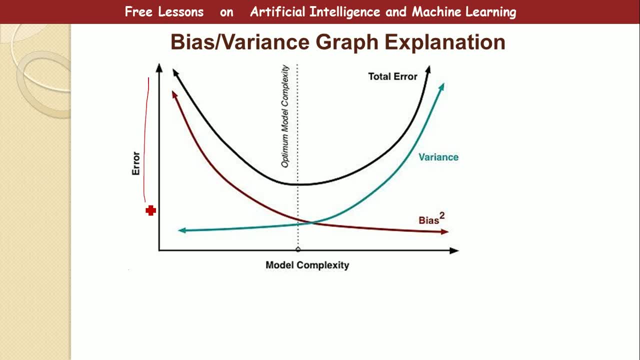 And the objective is to reduce this error to the minimum or to get it to come down. To get the error to come down, it means that, you see, let's look at the bias first, Or let's look at the variance first. 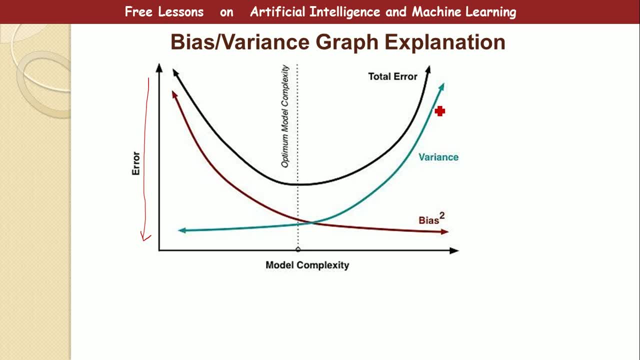 It means that we need to reduce the variance. Remember that. okay, we need to reduce the variance. of course, The variance has to come down. It has to come down, okay, and then along the line, it comes to this point. 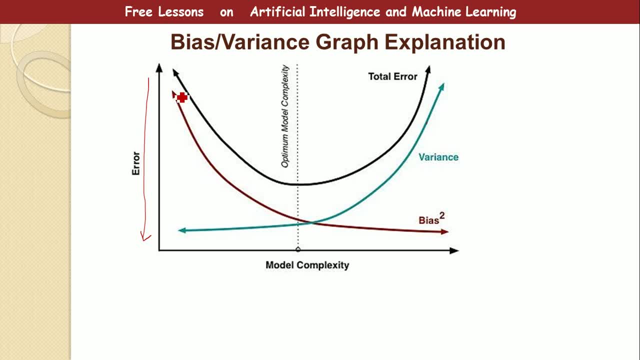 But as it's coming down, the bias is going up and the error is going up at the same time. So let's look at model complexity. When the model complexity is increasing, okay. when the model complexity is increasing, the bias is going down, the error is reducing, okay, which is very fine. 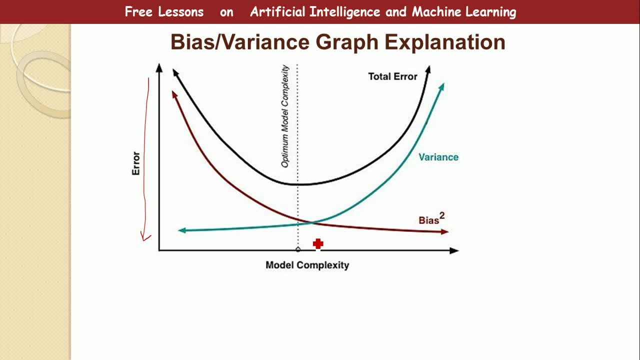 Okay, But at that point, the more you reduce the model complexity, okay. the bias becomes at the point whereby the error starts increasing again. So it means that there is a tradeoff point somewhere where the error is at its minimum, And that is where we have optimum model complexity. 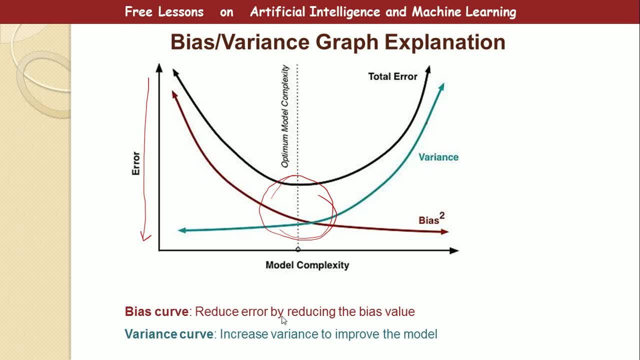 So we have that Bias curve: reduced error by reducing the bias value. The variance curve: increased variance to improve the model. So this is the variance curve. You move this way because you need to increase the variance so that the model is going to improve. 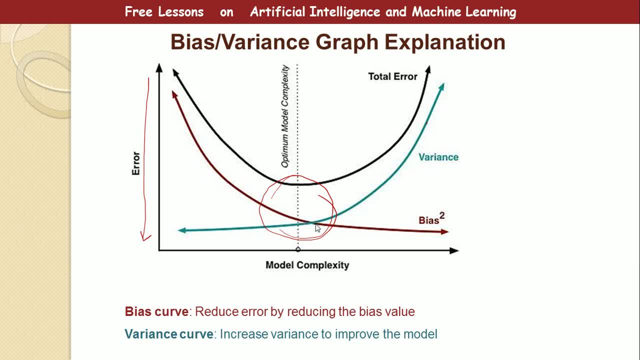 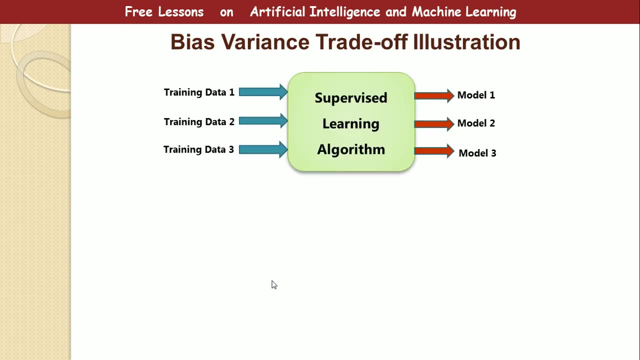 But if you get to this point, you are going to stop, because if you go any further, the error increases again. So this is how the bias variance graph works. If it's not very clear to you, take some time to go through it and look at the explanation. 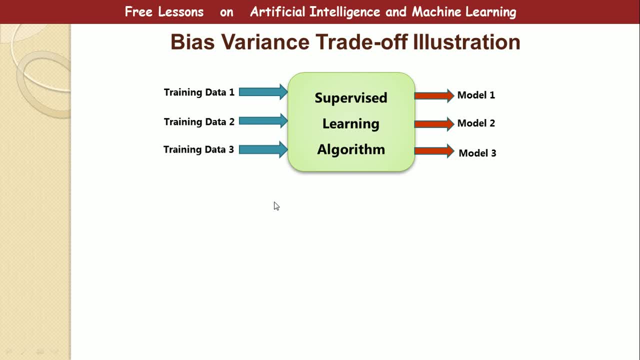 Let's now look at an illustration of how it works in real. We have training data sets, three training data sets that provide three models. These three models are based on the same algorithm, meaning that these three models are expected to perform the same way. 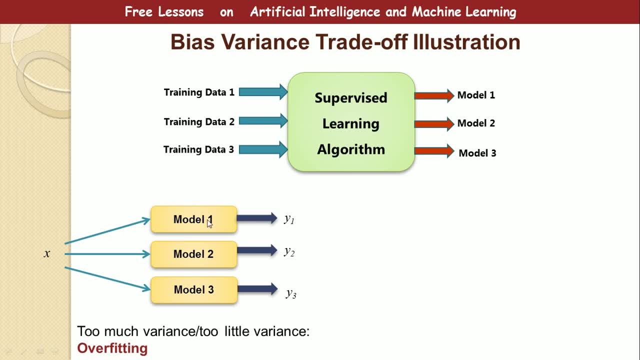 So good. So in the first case we have three models. Okay, So in the first model we have model 1, 2, 3, we're passing a value of x through these three models. We expect that these models provide the same output. but wow, this model provides a different. 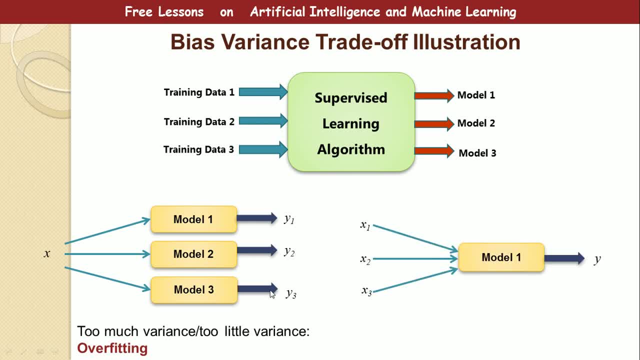 output. This one provides a different output. This model provides a different output. What it means is that these models have become too specific that it is not able to- it's not generalized enough to handle a new input. Okay, This is a problem of overfitting when the same algorithm provides different outputs. 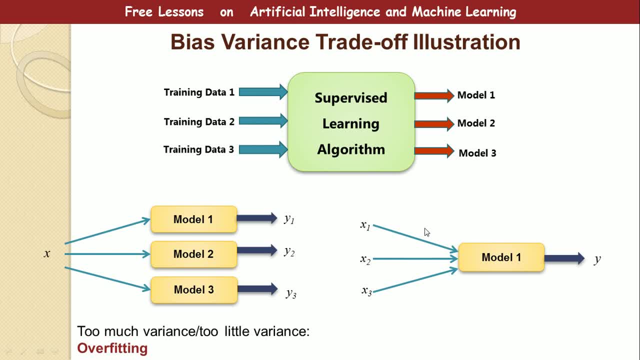 for the same imputes. Now let's look at a different case where we're passing three data sets, three different data, to a model of the same algorithm and these three data points, it actually should be able to provide different output. So in the first case we have model 1, 2, 3, 4, 5, 6, 7,, 8,, 9,, 10,, 11,, 12,, 13,, 14,, 15,, 16,. 17,, 18,, 19,, 20,, 21,, 22,, 23,, 24,, 25,, 26,, 27,, 28,, 29,, 30,, 31,, 32,, 33,, 34,, 35,, 36,, 37,, 38,, 39,. 40,, 41,, 42,, 42,, 43,, 44,, 45,, 46,, 47,, 48,, 49,, 50,, 51,, 52,, 52,, 53,, 54,, 55,, 56,, 57,, 58,, 59,. 60,, 61,, 62,, 62,, 62,, 63,, 62,, 62,, 63,, 62,, 62,, 63,, 62,, 63,, 62,, 62,, 63,, 62,, 62,, 63,, 62,, 63,, 62,, 63,.